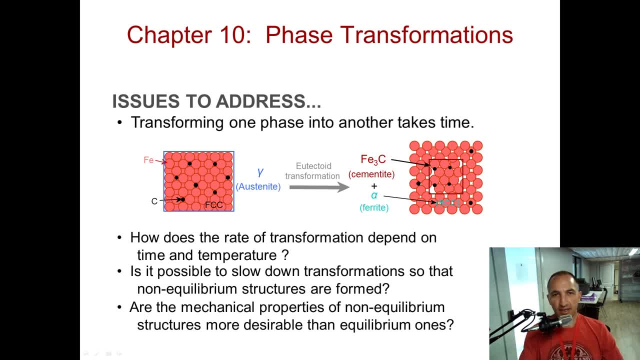 Good afternoon everyone. this is Eric Payton Introduction to Materials, Chapter 10, Phase Transformations. In this chapter we are going to address transforming one phase into another, which takes time. Here we have iron and carbon in the interstitials and that is an FCC lattice which is austenite. 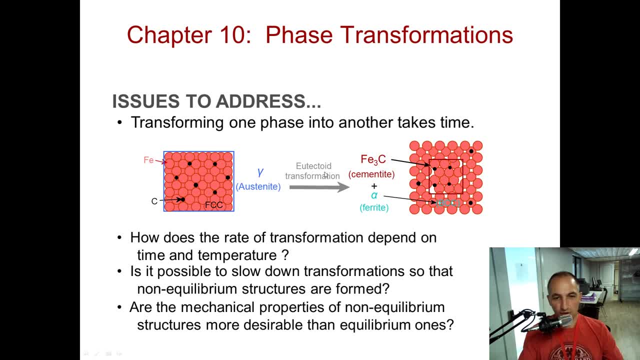 We also call that gamma. It goes through a eutectoid transformation as it cools and with that we have a second phase of iron carbide. We also call this cementite and alpha ferrite, which is BCC. The carbon is interdispersed in the cementite as this compound here. 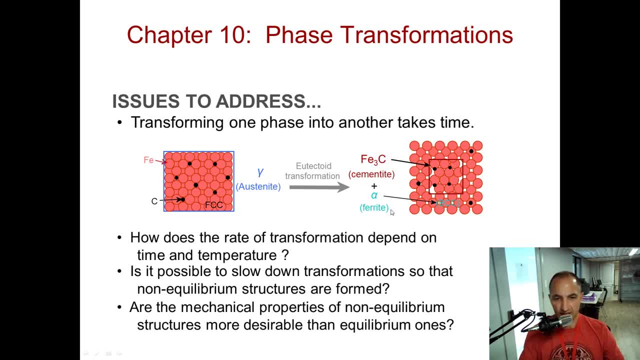 It is also a ferrite. It is also in the interstitial sites in the alpha ferrite. Also, we're going to address how does the rate of transformation depend on time and temperature? Is it possible to slow down transformation so that non-equilibrium structures are formed? 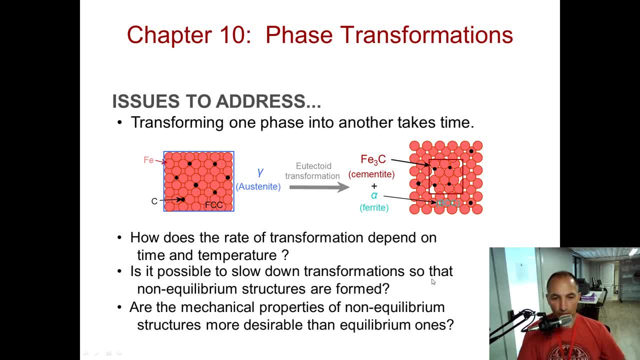 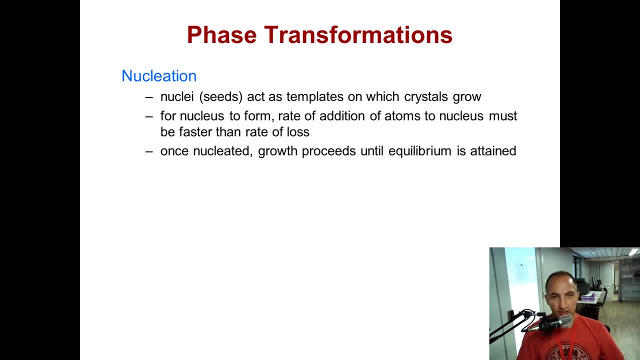 Are the mechanical properties of non-equilibrium structures more desirable than equilibrium structures? Phase transformations: Nucleation is the process where nuclei or seeds act as templates on which crystals can grow. So for nuclei to form, a rate of addition of atoms to the nucleus must be faster than the rate of loss. 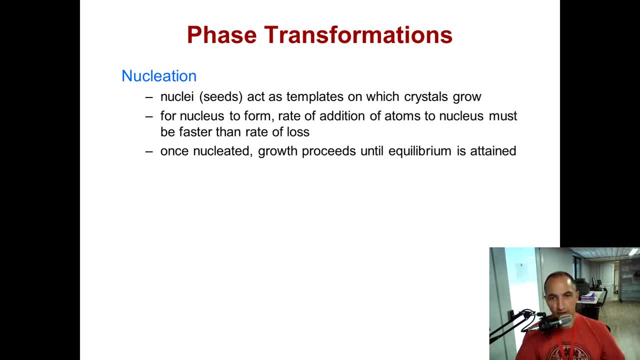 So there is this competing effect of adding atoms and then atoms dropping off. But once nucleated, the growth can proceed And proceed until equilibrium is attained And the driving force for the nucleation increases as we increase delta T. Delta T is also called supercooling. And. 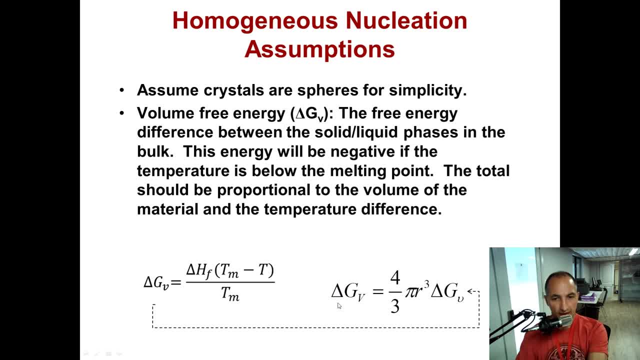 temperature of the material, and so by plugging in the Delta G on a per unit volume basis- and we know that the volume of sphere is equal to four-thirds pi arcs cubed- so that the total Gibbs free energy of that sphere is equal to Delta four-thirds pi arc cubed times the Gibbs free energy on a per unit volume basis. 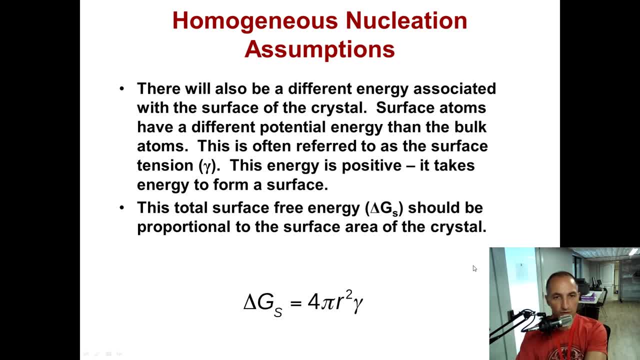 another assumption is that there will also be a different energy associated with the surface of the crystal surface. atoms have a different potential energy than the bulk. this is often referred to as the surface tension or gamma. but this energy is positive because it takes energy to form a surface. a surface has 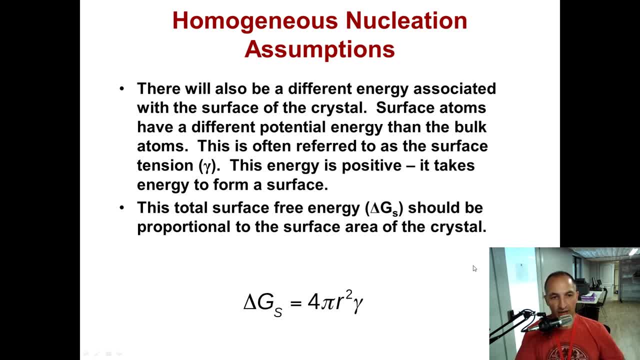 dangling bonds and so that that's why it requires energy for that. and this is the total surface free energy or Delta GS, and it should be proportional for the surface area of the crystal, which is four-thirds pi, 4 pi r squared. so 4 pi r squared times the surface tension is equal to our. 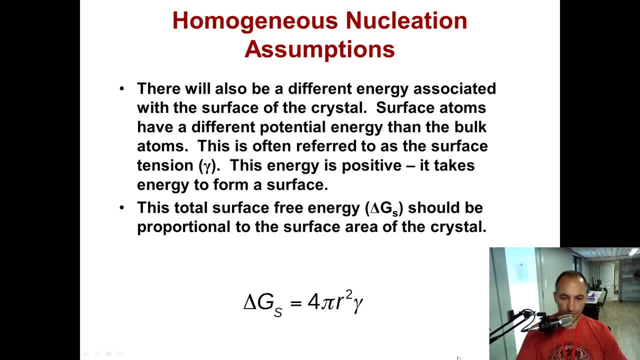 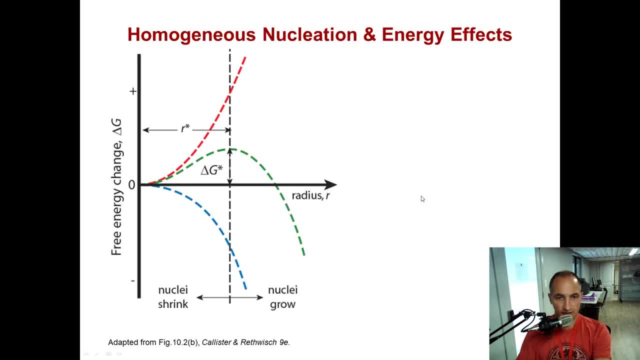 surface, Gibbs, free energy. all right, so there are these two competing effects. where I mentioned previously. we have the Gibbs- I'm sorry- we have the surface free energy, which destabilizes the nucleus because it takes energy to make this interface so that energy is positive, and that is equal to a 4 pi r squared gamma. 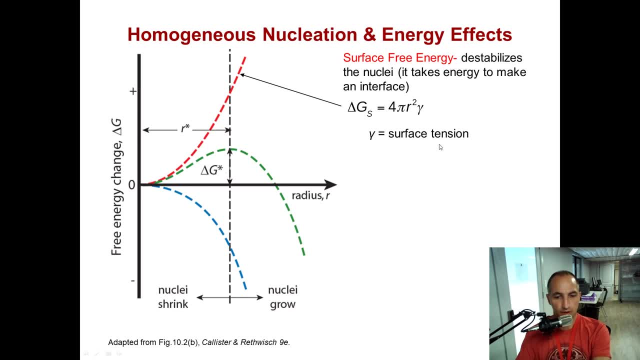 where gamma is the surface tension and we have the volume or volume of the surface tension and we have the volume or volume of the surface tension or bulk free energy, and this stabilizes the nuclei and so it releases energy. so the larger the volume, the larger the, the smaller the surface to volume ratio. so 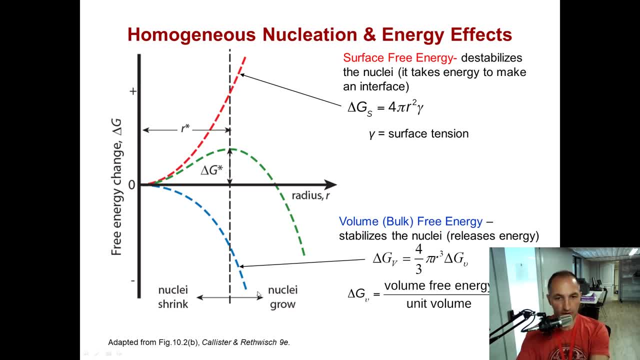 we have less dangling bonds on a per unit volume basis as the as the bulk free energy or as the radius of the nuclei increases. so remember that the, the bulk free energy is Delta GV equal to four-thirds pi R cubed times the Gibbs free energy. on a unit volume basis, Delta GV is equal to the volume free energy on 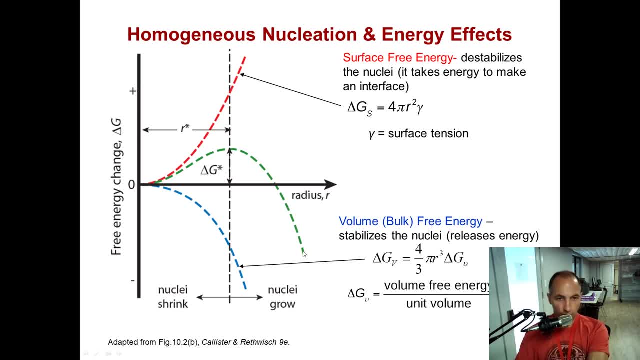 a per unit volume basis. what we need to do is the sum of this red and this blue curve is equal to this green curve. so initially the red is is the dominant factor, and then the bulk free energy takes over. so there is a Delta G star and there's also this R star. now, this is the, this is the. 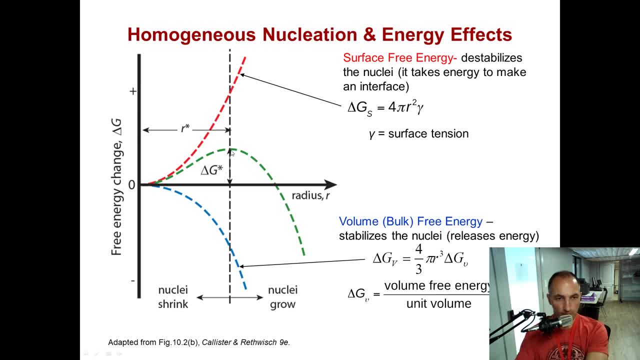 the point at which the slope is equal to zero. so you get, the slope is equal to zero. we take the derivative of this green line here. so we're going to be doing that. so we're going to be doing that on the next page. here, all right, and there is the total. free energy is just the sum of this term, and 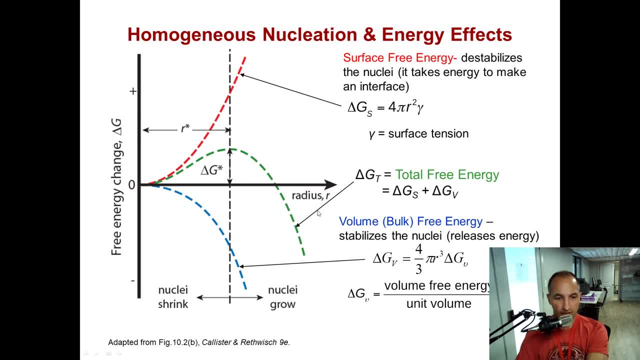 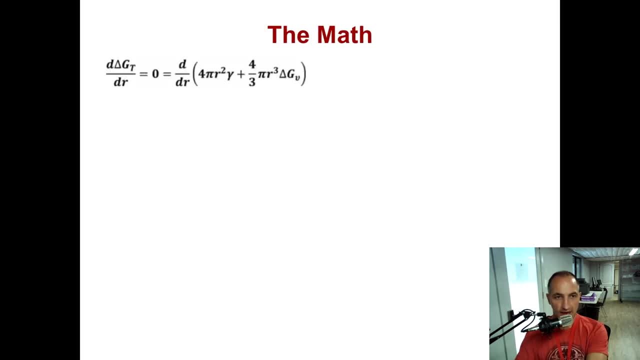 this term. so we add these two together and we take the derivative of that, and so the math here is that the surface term and then the volume term added together, the derivative of that is equal to a pi R. this is the critical nucleus. radius of the critical nucleus. 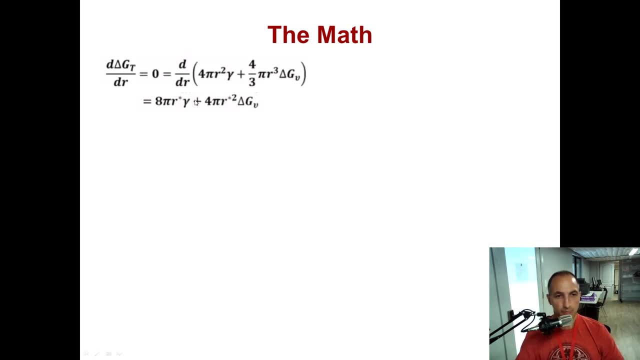 times the surface free energy plus 4 pi R squared times the Gibbs free energy on a volume basis, and so, solving for R star, we get negative 2 gamma over Delta GV, the. so from there we just plug that back into Delta G. T is the total Gibbs free. 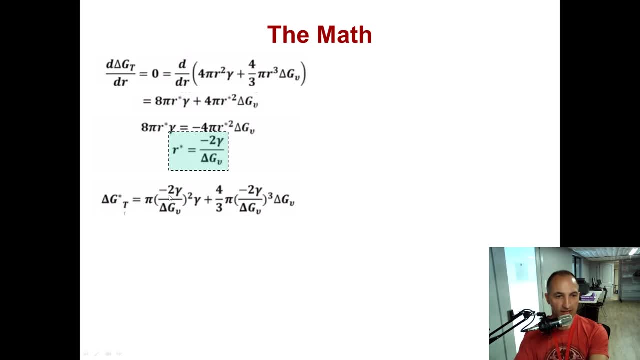 energy. so we plug it into here and we also plug R star into the second volume term and then we simplify and we get 16 pi I gamma cubed over 3 Delta GV in watt squared. now what we do is remember that the Gibbs free energy on a per unit. 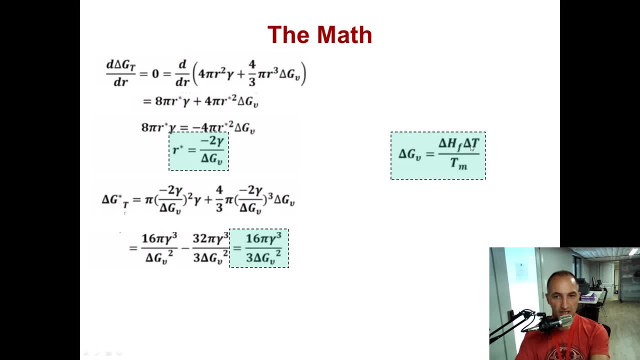 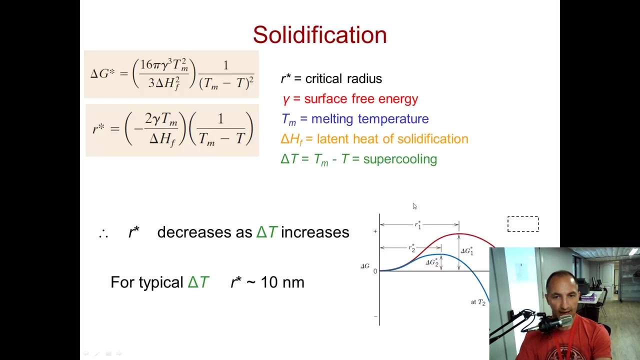 volume basis is equal to the enthalpy of formation times, the super cooling or Delta T over the melting temperature, and plugging that back in to the R star and also for the Delta G, the total Gibbs free energy, we can get these final two terms. so this: these are the solidification terms for homogeneous 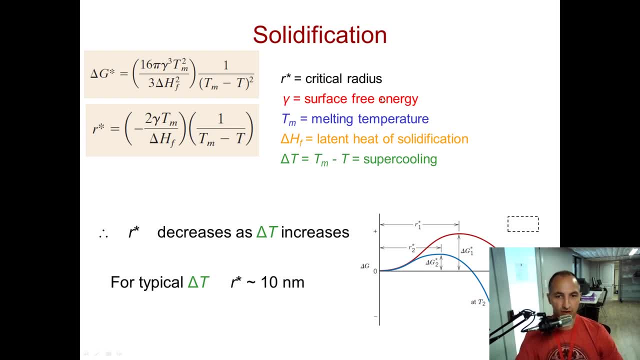 nucleation. remember R star is the critical radius for the nucleation. gamma is the surface free energy. Tm is the melting temperature. we have the latent heat of solidification and the temperature of the melting temperature and the super cooling or Delta T. therefore the R star decreases as Delta. 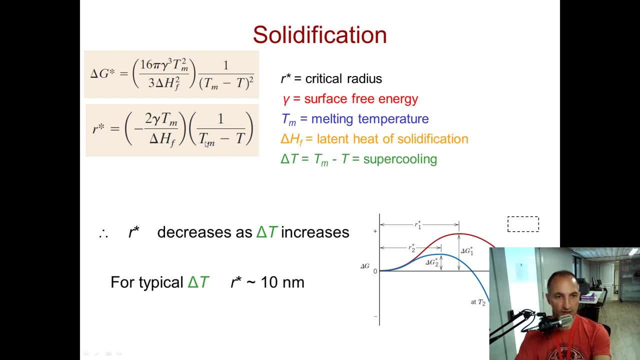 T increases as Delta T increases, here we get R star decreasing. and down here on the right you can see two examples of a larger R R star and a smaller R star. smaller R star is also a smaller total of Gibbs free energy. so also to note here is the latent heat of solidification and gamma are weakly. 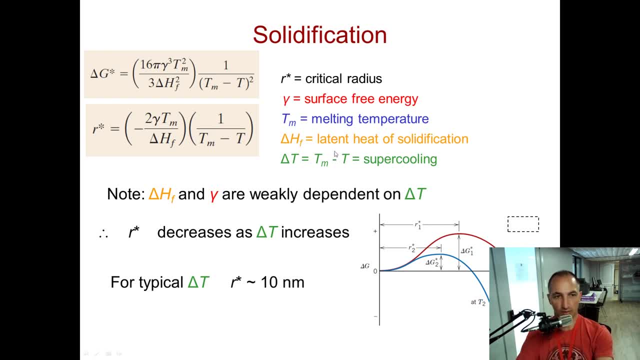 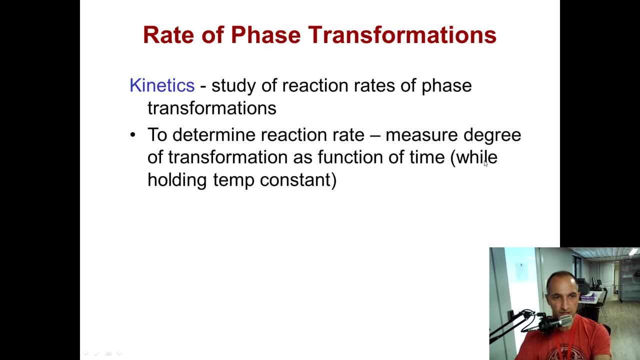 dependent on temperature. so and pull those out from the equation. the the rate of phase transformations is also called kinetics and the study. the kinetics is the study of the reaction rates of phase transformations and to and to determine the reaction rate, we have to measure the degree of transformation as a. 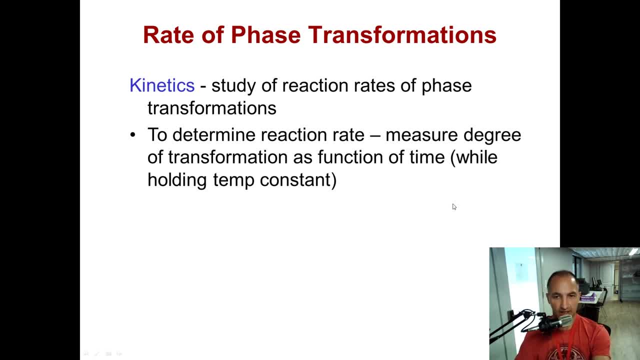 function of time while holding T constant. so that's the final method for measuring the degree of transformation. so how do we measure a degree of transformation while it's being cooled? there's several techniques here. one is x-rays of fraction, and this requires many, many specimens. you have to have a 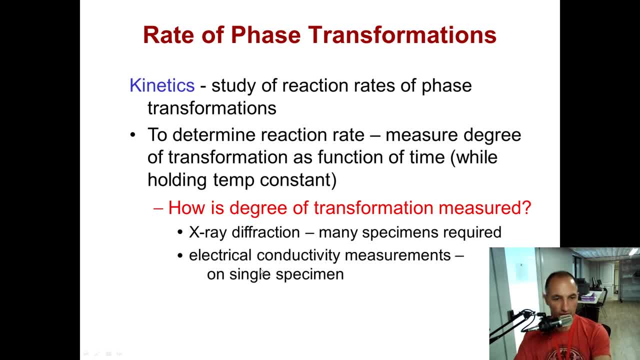 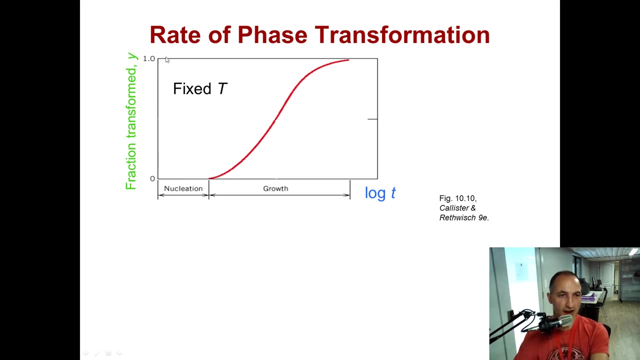 different specimen for each cooling rate and another method, for example, would be phase. another method which only requires a single specimen is electrical connectivity, as the connectivity changes as the phases change, or measuring the propagation of sound waves, and this is a graph here showing the fraction transformed on the y-axis and 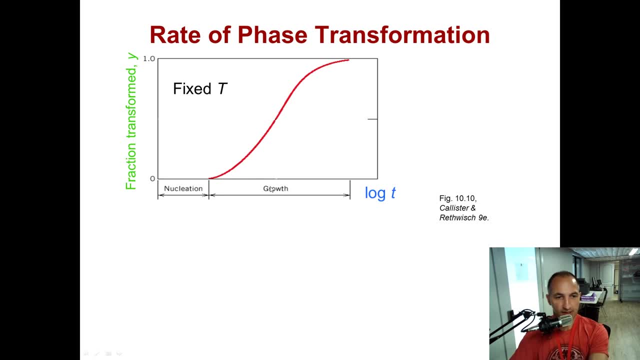 log of time on the x-axis. so there's this point prior to nucleation. before we can get to an R star or critical nucleus, we have no transformation. and then, once we start forming nuclei and they start to grow stable, then we start to see growth and initially it's very rapid and then it reaches an inflection here where 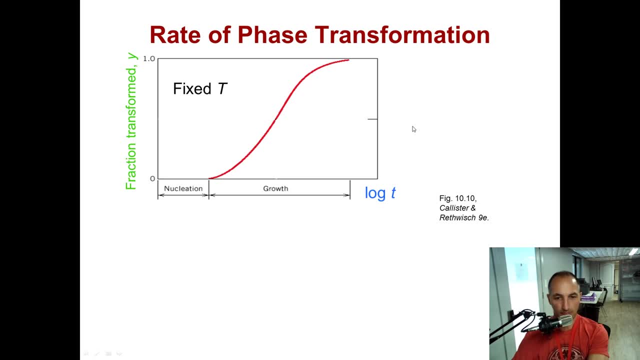 it start, the transformation starts to drop off again and the the rate increase increases, initially as the nuclei grow and it reaches a maximum rate and transformation is complete at the top. and this is all at a fixed temperature below the equilibrium temperature. so this is at a supercooled temperature and we're holding it at that temperature. this is 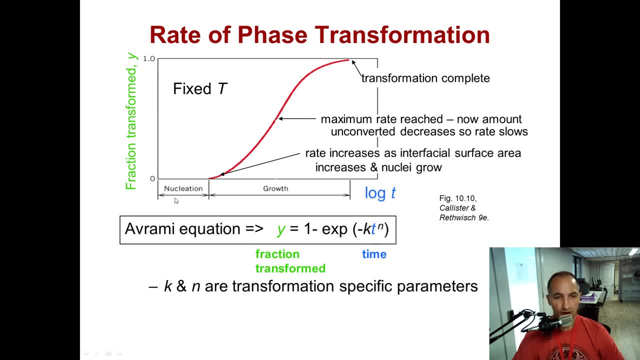 called the Avrami equation. the Avrami equation, as the equation y is equal to 1 minus e, to the negative, k, T, n and k and n are transformation specific parameters, so the that will be the rate, or you know how steep this is, and also 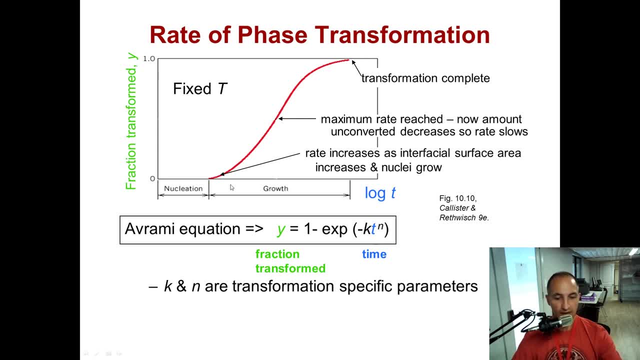 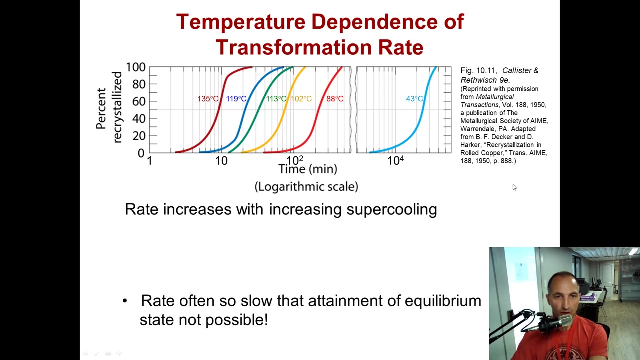 the point at which it starts to nucleate and grow. so the half way transformation is by convention. we calculate that as the rate. so the time at which you have 50% transformation, take one over that and that's what we call the rate of transformation. so now, if you look at these Avrami curves- all where we holding the 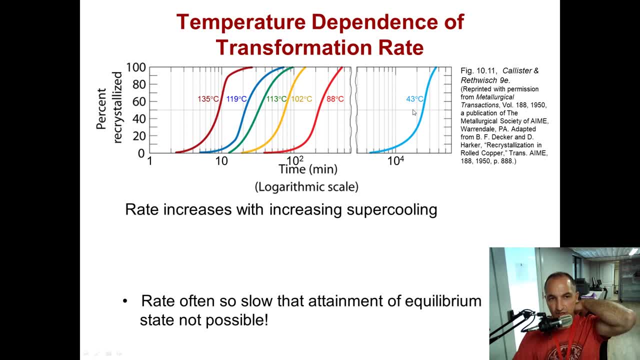 temperature. at different temperatures below below equilibrium, we can see that the rate will increase with the degree of increase super cooling. so the graph on the left here has the highest amount of super cooling: 135 degrees of super cooling. that's our Delta t and with less Delta t it takes longer to nucleate and 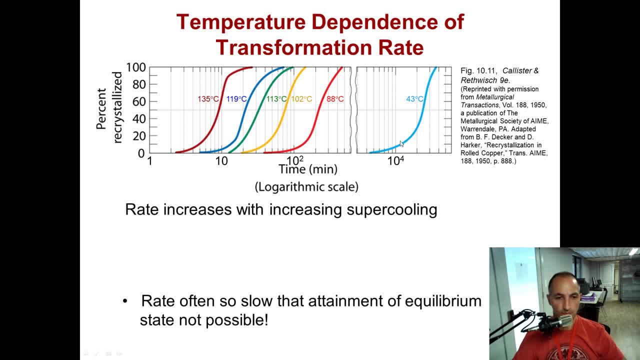 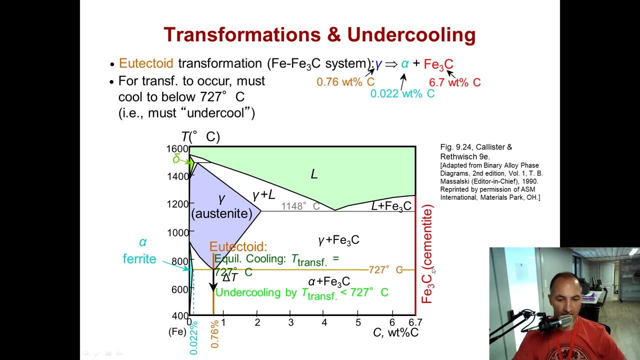 it takes longer to transform. the rate is often so slow that attainment of equilibrium isn't possible. now this is the iron-carbon phase diagram, and we're going to review this for you so that you can break it down in just a couple of minutes if we want to. 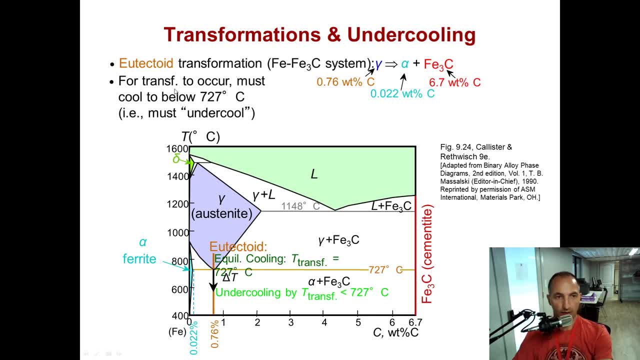 this is something that you've seen before, but and you've been introduced to the term eutectoid transformation. remember, this is one solid going to two other solids, so in this case we have gamma iron transferring to alpha iron, plus iron carbide or cementite, and the carbon concentration of gamma is point. 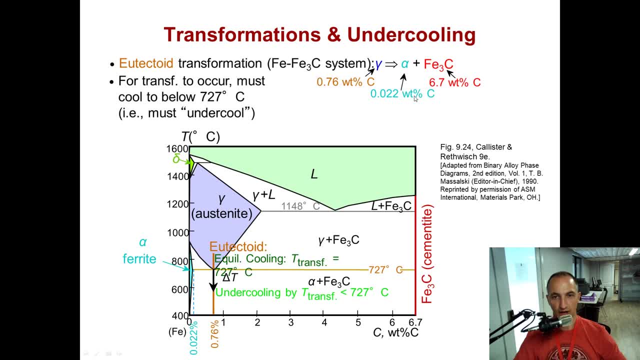 seven six, and the concentration of carbon in alpha is only point zero, two percent, and iron carbon is very high at six point seven. so here's the six point seven percent for the iron carbide or cementite and the, the gamma, which is right here, at point seven six. so we're cooling at the eutectoid temperature. which is, I'm sorry, the eutectoid composition, which is point seven, six percent carbon, and as we transition below 727 degrees C, we're starting to under cool and the transformation will then occur at some temperature below 727 degrees C. so what's the difference between eutectoid and carbon? 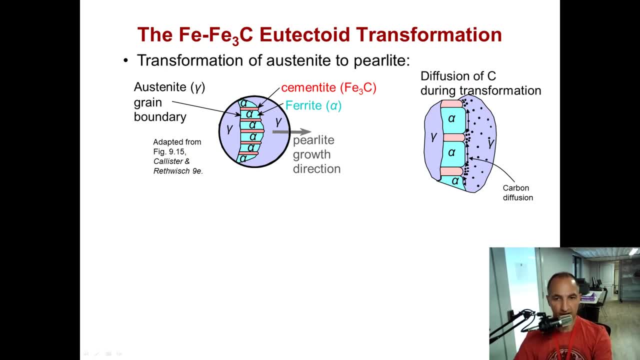 happening at the closer, at a finer scale here, as we're cooling at this eutectoid composition. what's happening here is that we start out with all austenite and at the austenite grain boundary we start to get nucleation of the. so this is heterogeneous nucleation, because at the grain boundary start to 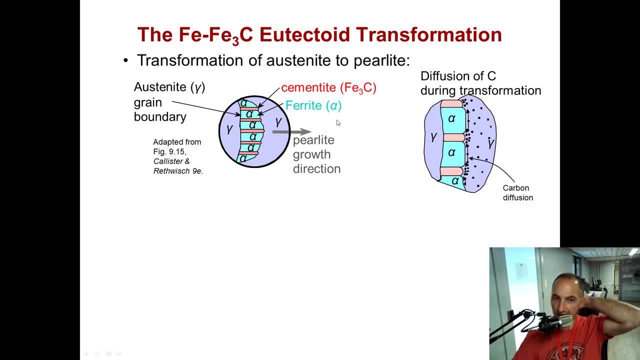 get cementite and alpha iron or ferrite growing and it grows in these platelets and we call those platelets pearlite. so the pearlite growth direction is to the right here. if you zoom in on that and look at that even closer, what's your, what? 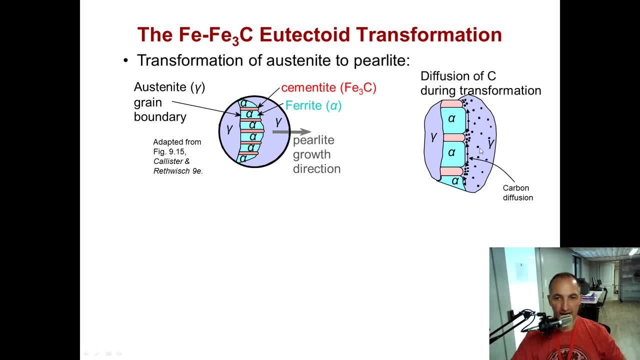 you find here is that the carbon that's in the austenite has to diffuse in theseedanite soils to get emotionally distilled and debuted again. so how browned fatty iron residual understand the first term of carbon is to the second, here and here and then. here we're easy to absorb and then when he find out where ostenite is still active for about 10 to 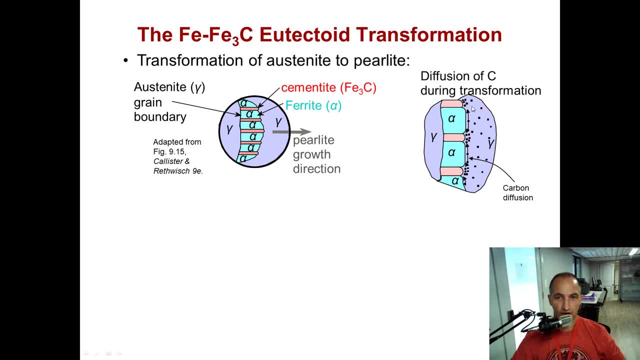 minute. our measurement will be pretty basic, reversing this step of absolute nothing. it is really just Building up of the or away from the ferrite, because that has a carbon concentration of only 0.02% and it it has to then migrate over to the high carbon composition phase. 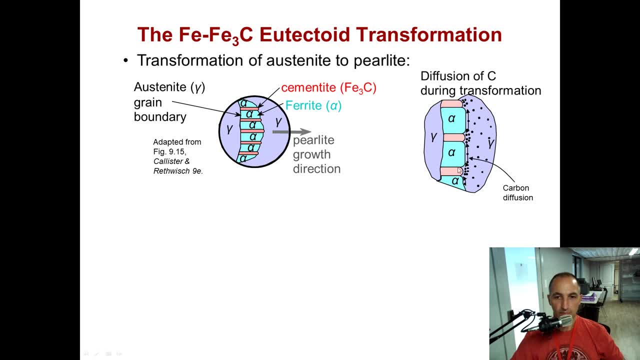 which is the cementite. so the, the movement of the carbon occurs in the liquid austenite. I'm sorry, it occurs in the, not the liquid. it occurs in the austenite, and so the faster this growth occurs, the finer these platelets become, because the carbon can't diffuse as much. 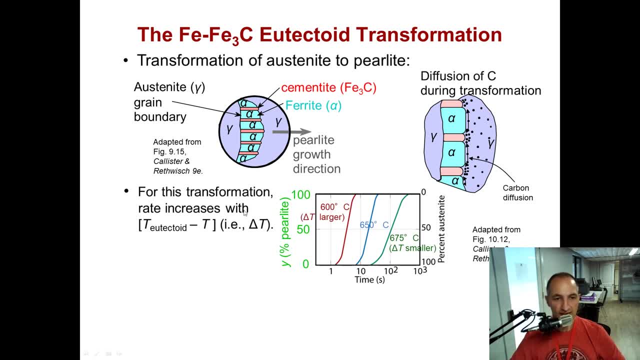 so for this transformation, the rate increases when you have a Delta T of greater and greater. so this is a Delta T of- I'm sorry, this is the actual temperature here- of 600 degrees C, and so that's the highest amount of super cooling because, remember, the eutectoid temperature is. 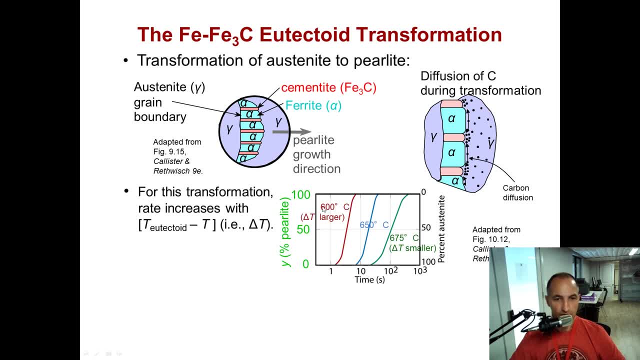 727 degrees C. so that's 127 degrees C Delta. now at less super cooling or under cooling. the rate of transformation takes longer and longer, so that has a smaller Delta T going to the right. what I alluded to earlier is that you have different types of perlite than 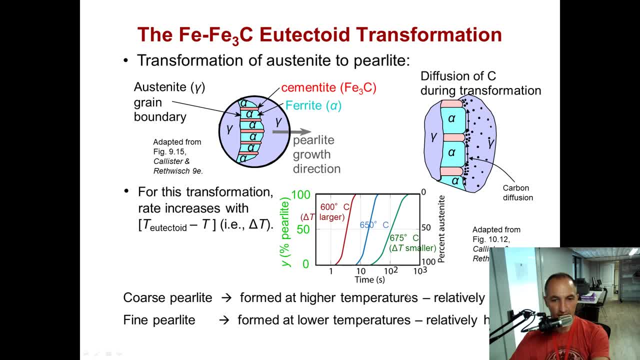 forming. you have a coarse perlite which is forming at higher temperatures, where you have a smaller amount of under cooling, and that's relatively soft. and you can have fine perlite which is formed at starter temperatures, whether it's a boilingOl at lower temperatures or more super cooling, and that's relatively hard. and 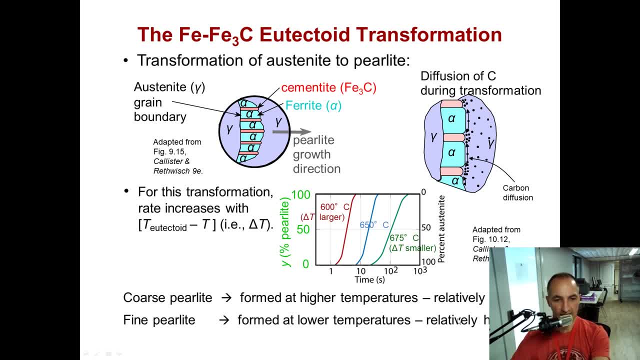 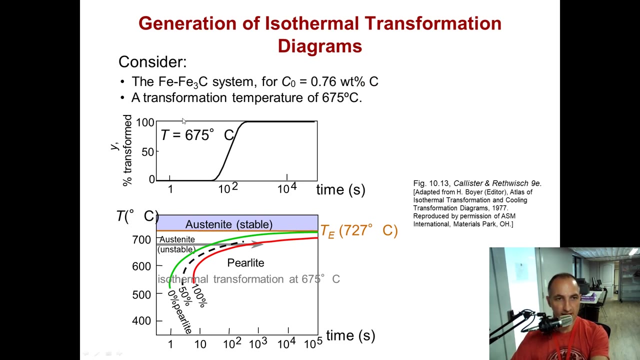 if you recall, back when we looked at the case study of the Titanic, there was the Titanic had a coarse pearlite and modern 836 eels have a fine pearlite. so let's look again at the Avrami plot and taking a step back now, and here's the 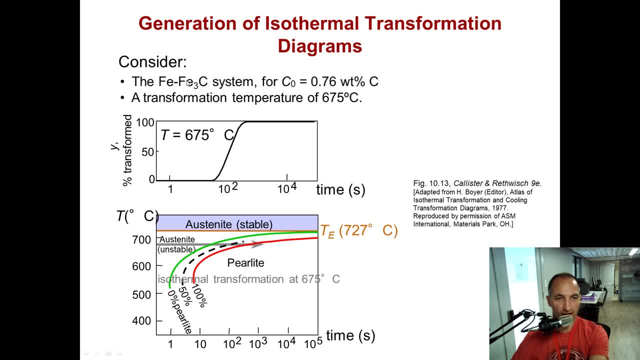 Avrami curve or the iron carbide system at the eutectoid opposition. so the overall composition of 0.76 weight percent carbon and a transformation temperature of 675 degrees C. so this remember that eutectoid temperature is 727, so we're super. 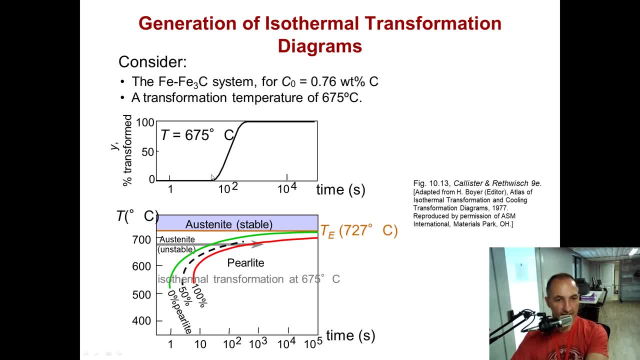 cooling it and it takes a certain amount of time before we can start nucleating and having stable growth of the pearlite and then we get a hundred percent transformation. so, on the Avrami plot, what we, what I'm introducing down here on the on the graph below, is: 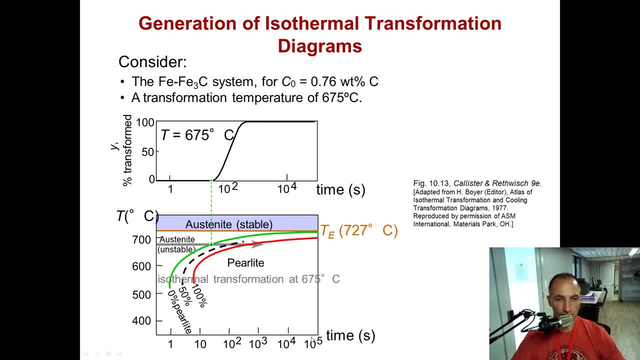 called a transformation diagram, and transformation diagrams allows us to take a whole bunch of these Avrami plots and create just one transformation diagram. so that is extremely helpful because you don't have to have Avrami plots, hundreds and hundreds of Avrami plots, all for different compositions of 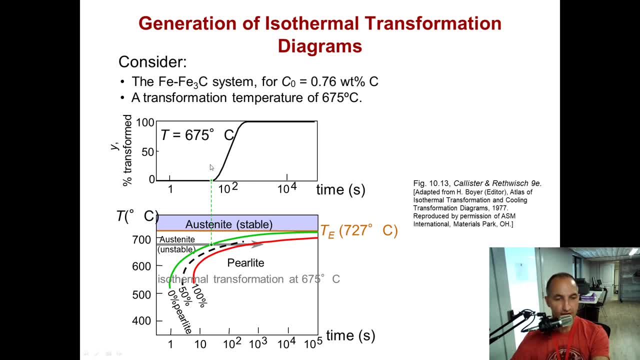 of carbon and at different amounts of super cooling. so there is the green line is when we first start to get a nucleation and growth of pearlite and we achieve 50% transformation of pearlite at the dotted line here and we achieve a hundred percent transformation at the red line here. 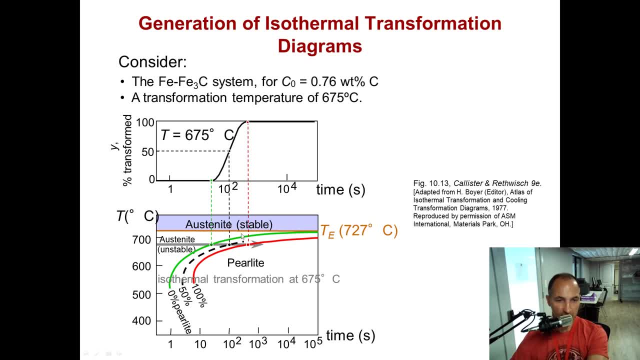 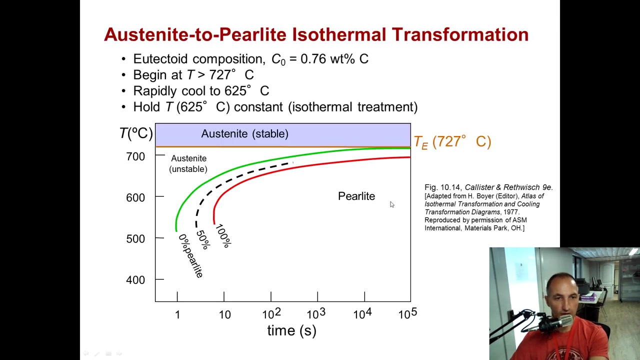 where it exits this transformation band and goes into 100% pearlite. so this is the isothermal transformation diagram, or holding at 675 degrees C. all right, so in this blue area here we have stable austenite again. this is at the eutectoid. 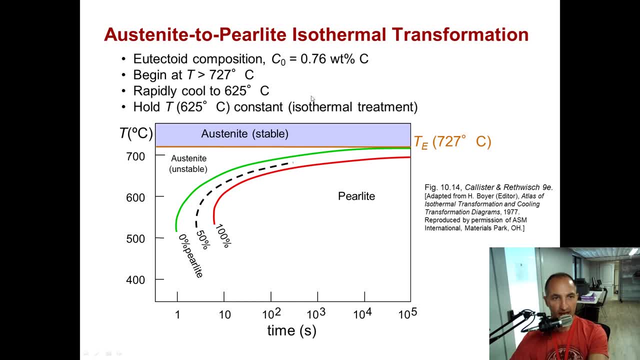 composition of point seven, six weight percent, and we begin at a temperature that's greater than 227 BC, and then we rapidly cool to 625 degrees C and then hold at 625 degrees constant temperature. so that's what we call it, the isothermal treatment. so 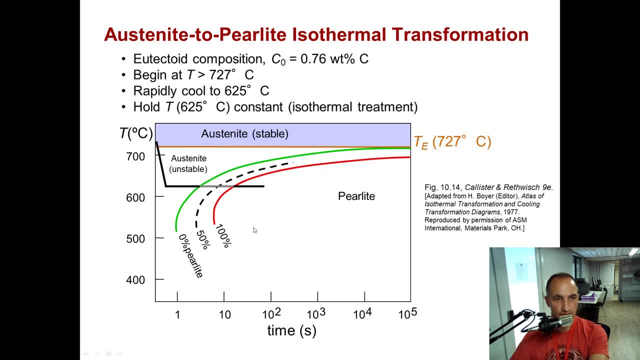 let's draw that line. there is where we're quenching it and here is where we're holding it. so in this light gray area is when we're transforming the unstable austenite into stable pearlite. so if you were to look at the microstructure of point right when it 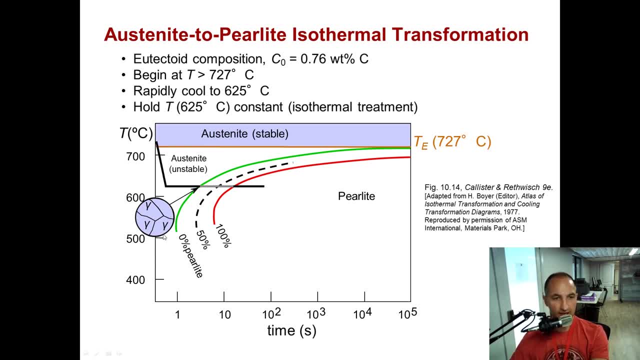 starts to transition. we have all austenite grains and then, at 50%, the pearlite has nucleated along the grain boundaries of austenite and grown and then. so these zebra stripes are the alpha and iron carbide, lamellae and a hundred percent transformation of pearlite as it exits that band. 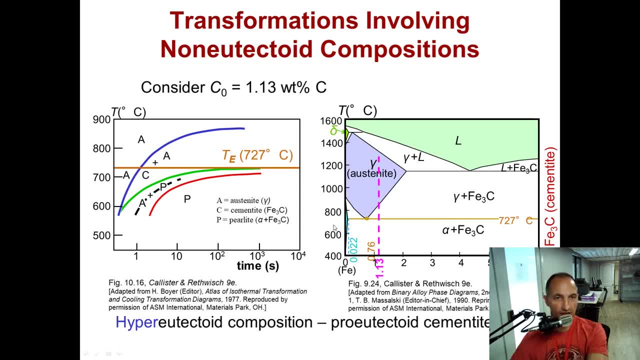 so transformations involving non-eutectoid compositions get a little bit more complicated, but not too much. you have, and we've done, some shorthand here, where A is austenite or gamma and C is cementite and P is pearlite. what we've done here is we've quenched to, or this is: 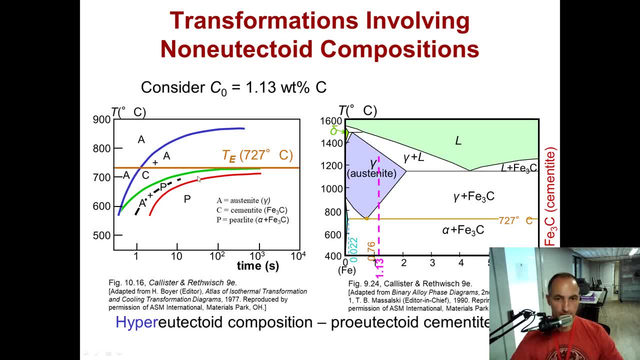 the 727 degree C. so this is the eutectoid temperature. and now we're looking at one point one: three percent carbon, which is this pink dotted line here. so we're on the right side of the eutectoid stopped carbon, which is this pink dotted line here. so we're on the right side of the eutectoid side and we're on to neutral. צרff, Godzillastarb, resТыc, sweatервh. 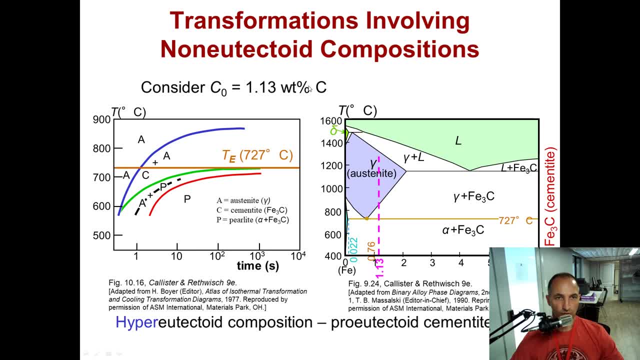 composition of 0.76. so that's why this is called a hyper eutectoid composition, as it's higher than the eutectoid composition, and that means we're going to have pro eutectoid cementite over on this side. remember, this is hypo on the 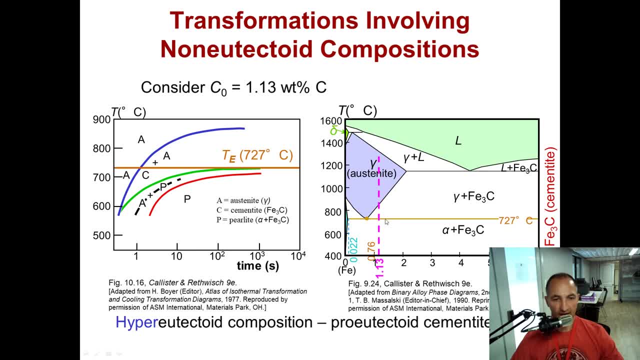 left side hyper eutectoid and then on the right side is hyper eutectoid compositions, and on the left side you'll have a pro eutectoid as well, but you'll have pro eutectoid alpha, and on the right side you have pro eutectoid. 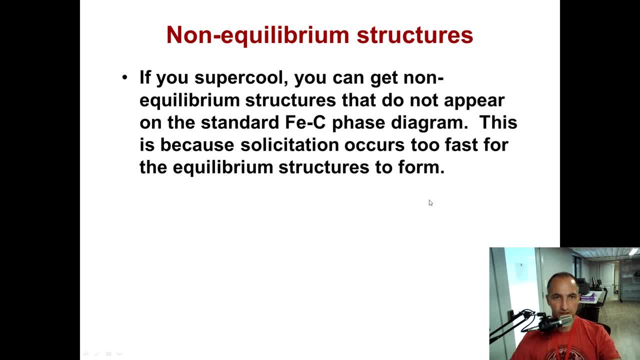 iron carbide. so let's look at the non equilibrium structures. so if you super cool, you can get non equilibrium structures and they don't appear on the standard iron carbide phase diagram and this is because solidification occurs too fast for the equilibrium structures to occur. 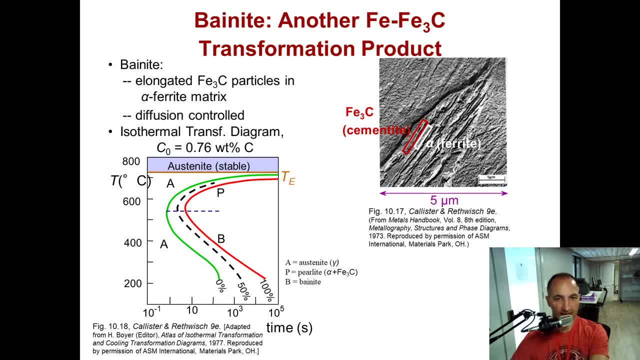 now here's what one of those phases looks like. on the right it's called bainite. a bainite under electron microscopy- or yeah, this is an SCM- will have a non equilibrium function and that's okay, because you'll have your bainite. have these fine platelets of iron carbide next to platelets of of the low. 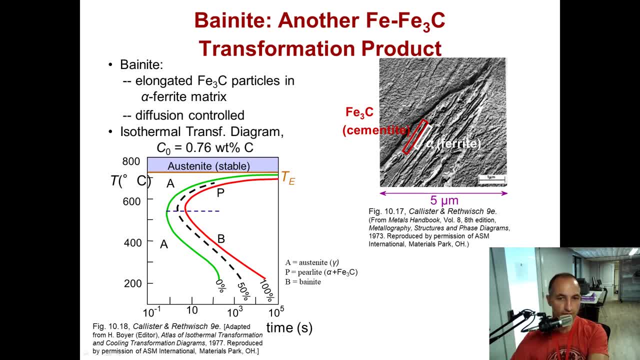 carbon composition, alpha iron or a ferrite. so the bainite are elongated iron carbide particles in this alpha ferrite matrix and it's diffusion controlled. so if we were to do an isothermal transformation diagram looking again at the overall composition of 0.76. so this is the eutectoid. 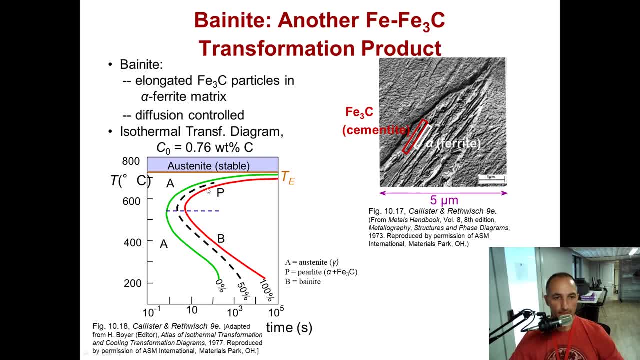 composition of 0.76 and we can see that above the nose of this isothermal transformation we have pearlite and below that nose we have this B, which is this other phase here, which is bainite, and you can- it's below here because, see, this is more super cooling. we were to 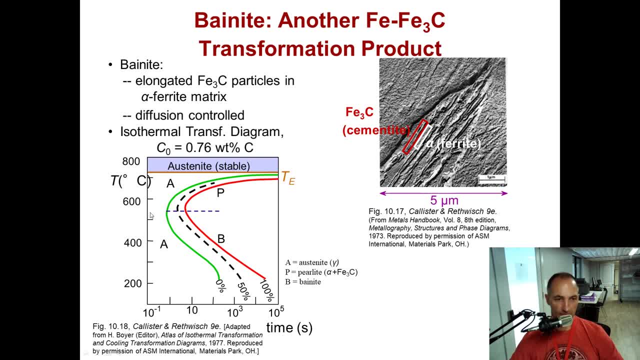 quench down below, you know, 525 degrees C or whatever, you could start to get some of this other phase here, bainite. so if we were to cool, to rapidly cool, to 600 and hold, we'd get 100% pearlite and you, and if we were to rapidly cool to say 475 and hold, we get 100% bainite. 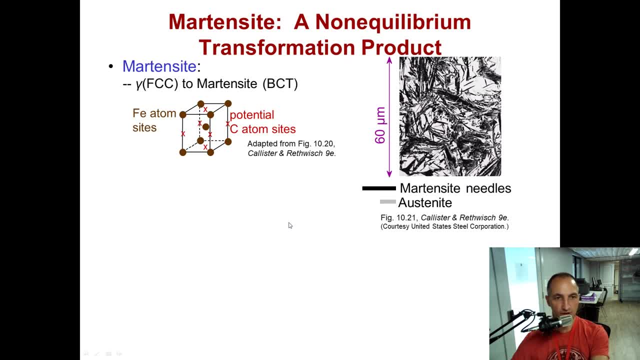 another non equilibrium transformation product is called martensite. now, martensite is this transformation from austenite, the gamma, which is an FCC crystal structure, to martensite, which has a body centered tetragonal structure. so the it doesn't have enough time to transition to a BCC or body center. 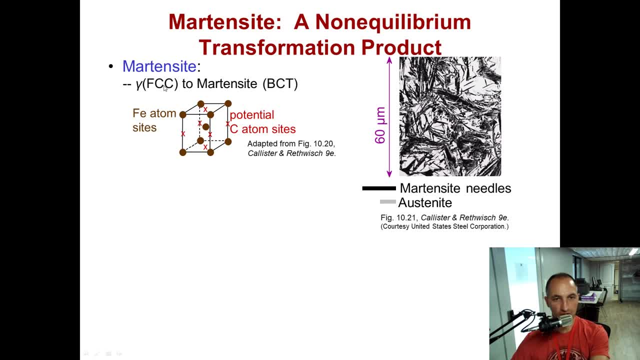 tetragonal, which is normally the low temperature base or, I'm sorry, crystal structure. so the, the carbon atom, doesn't have a chance to leave the lattice, or two diffused out of the lattice, so gets locked into the lattice and it so stays like an FCC arrangement of iron atoms, but it becomes elongated, because now it 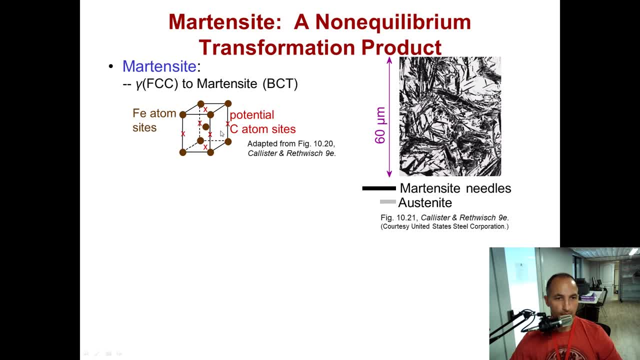 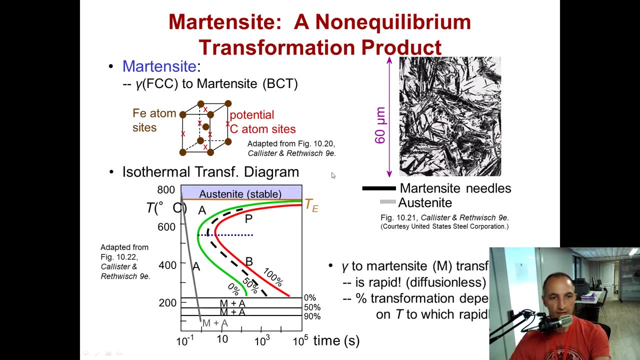 has these carbon atoms that are shoved in there which prevent it from obtaining its true FCC crystal structure. and this is what it looks like: these little whiskery needles of martensite. now let's look at the isothermal transformation diagram for austenite at the eutectoid composition. we would 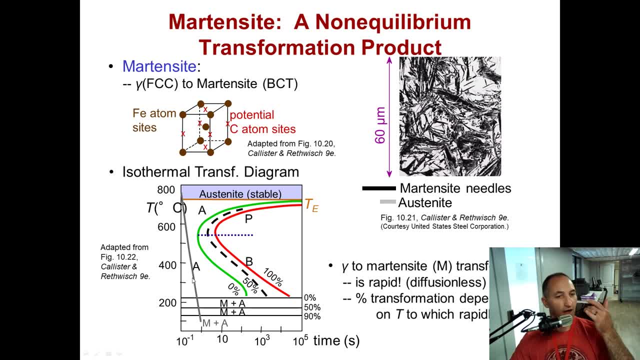 have to rapidly quench all the way down to get martensite. and so this is this light gray line here, going all the way, starting with zero percent martensite, fifty percent martensite and then a hundred percent martensite. M stands for martensite, A stands for austenite. here. 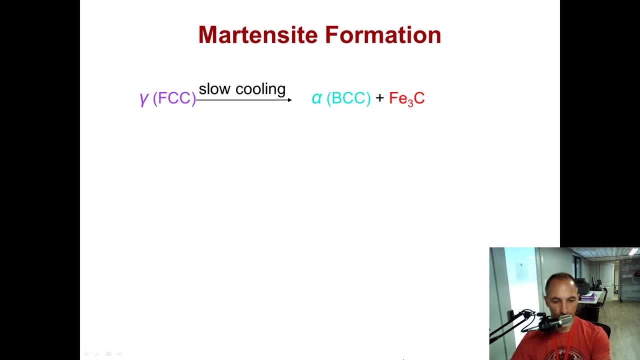 so let's look at the martensite transformation we're starting with with gamma iron, which is, or austenite, which is FCC, and if we slowly cool that, we get the ferrite, which is BCC and iron carbide. but if we were, if we quench it, 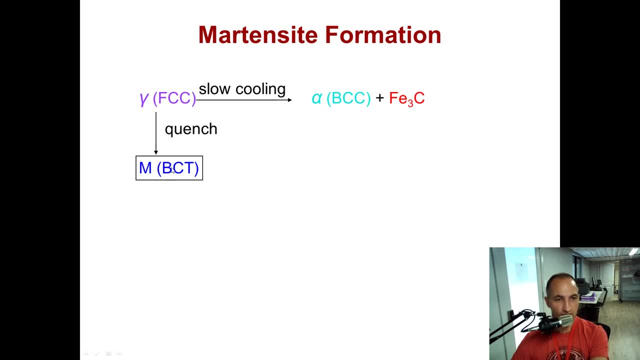 instead we get martensite, which is a body centered tetragonal structure and so the martensite is a single phase and it has this bct crystal structure and it's diffusionless. and these, this bct crystal structure, has very few slip planes, so it's extremely hard and brittle, don't have a lot of dislocation motion. 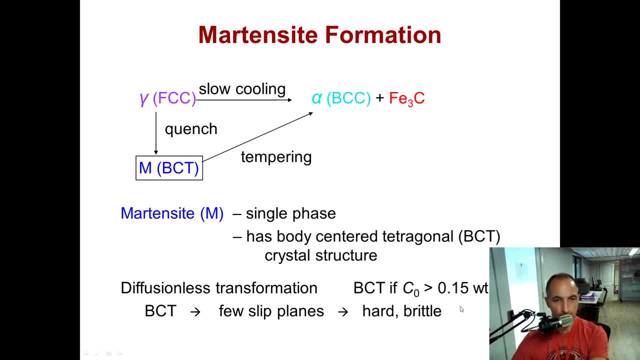 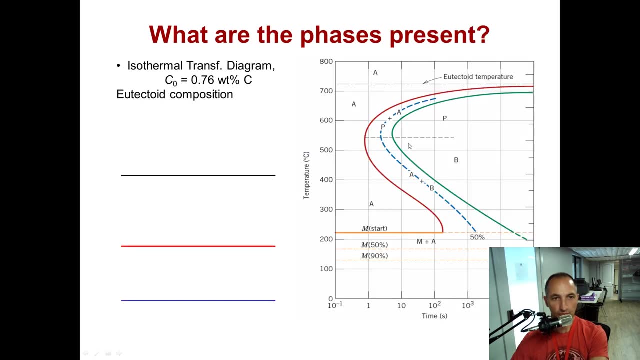 and not much ductility. so what we do instead is we can temper martensite, which is a high temperature thermal treatment, and we can get back to the alpha plus Fe3C. so let's look at, let's look at an example here of the eutectoid composition of 0.76 weight. 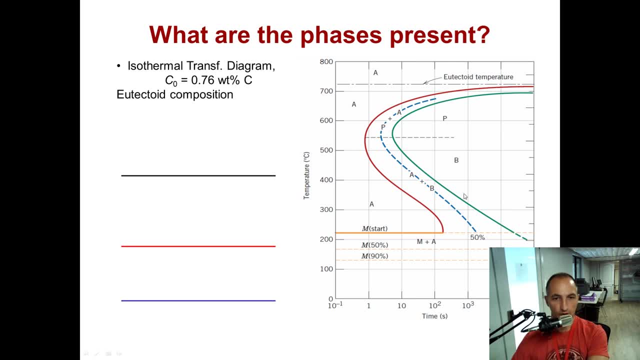 percent carbon and we're going to do a couple of different thermal treatments. the first one is to rapidly cool the 700 degrees C and hold for 10 to the 4 seconds and then quench to room temperature. let's do that, this. that's the black line here: 700 degrees C. we're below the 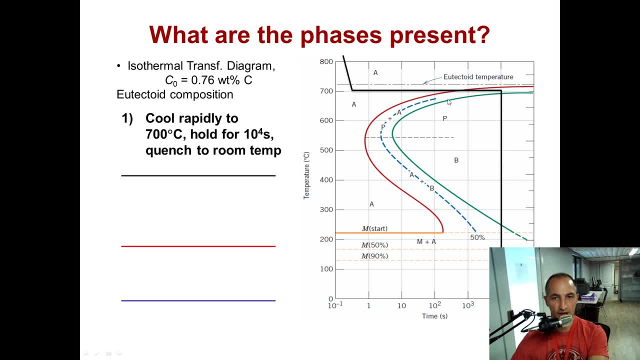 eutectoid temperature and it's taking a long time, but eventually we start to nucleate perlite and then we rapidly quench. so there we're going to get a hundred percent perlite. the second one is we're rapidly cooling to 400 degrees C, so this is much higher under cooling or super cooling, and we're 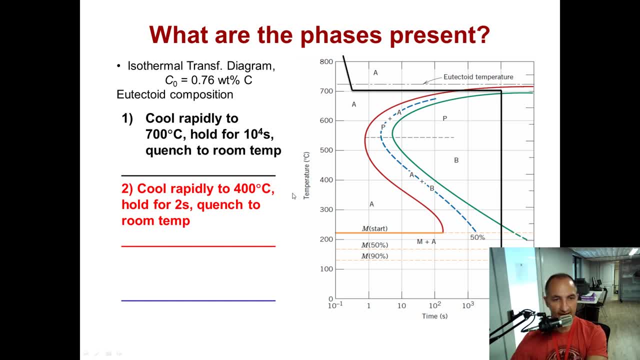 holding there for two seconds and then we're cooling to 400 degrees C and then we're holding there for two seconds and then we're quenching again to room temperature. so that's the red line, and there is the hold for two seconds and then quenching again. so from that it looks like we're 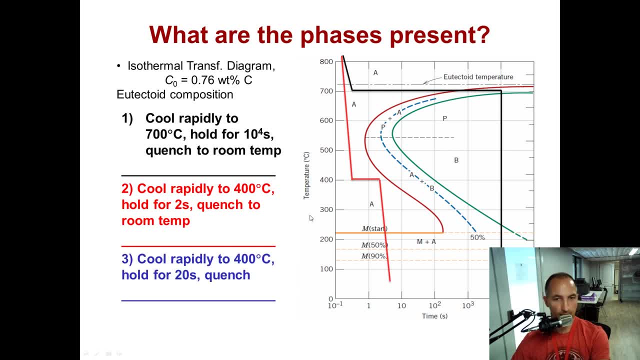 going to get a hundred percent martensite from doing that. now in the third one we're rapidly cooling to 400 degrees C and then we're holding for 20 seconds and that's this blue line here. so we're getting probably 25% transformation of the austenite to bainite and then when we 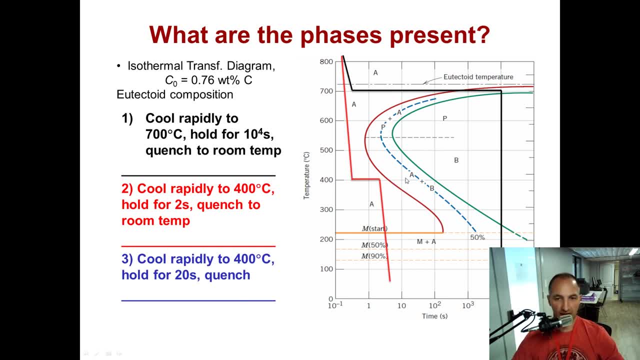 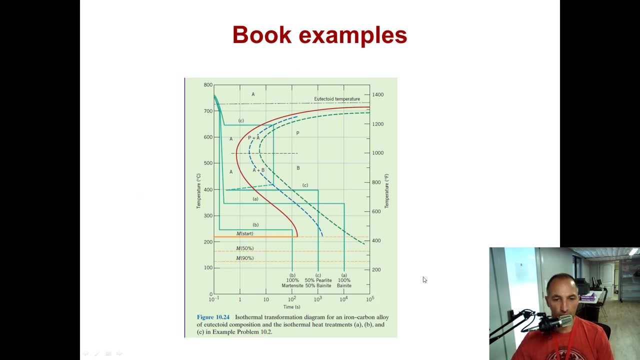 quench. the remainder, or 75% of the remaining, 75% of remaining austenite is left. it's going to form martensite. so there's several other book examples that will end up probably doing these in class, but you should also look at those. 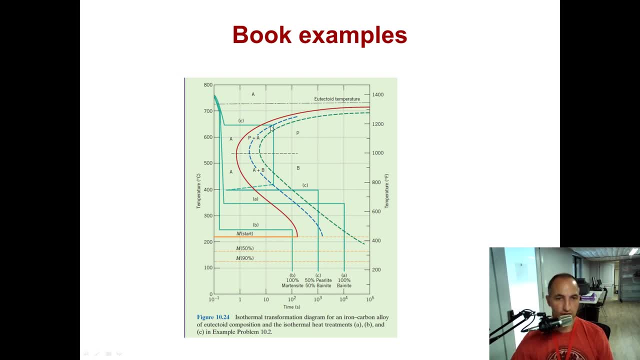 some of those where you're. you're going, you're maybe nucleating about 50% perlite and then you're quenching again and then holding it and then forming bainite for the rest of it. so that's the 50% perlite and 50% bainite. that's the kind of the 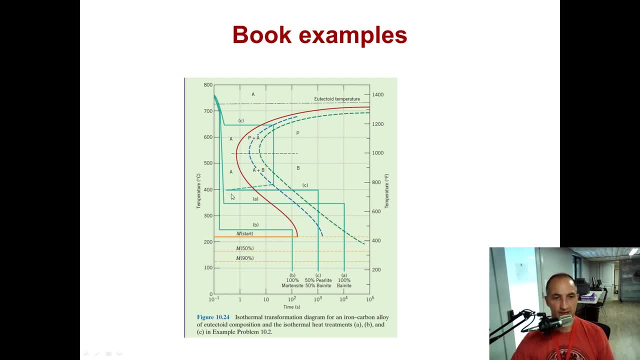 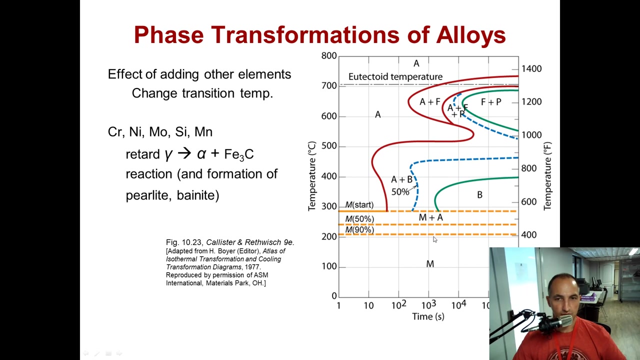 weird one, because you're sort of like going back in time and then this is the whatever remaining, austenite is left and is used to convert to bainite, and then other things you can do to modify the isothermal transformation is the addition of alloying elements. so what that does is it pushes all of these. 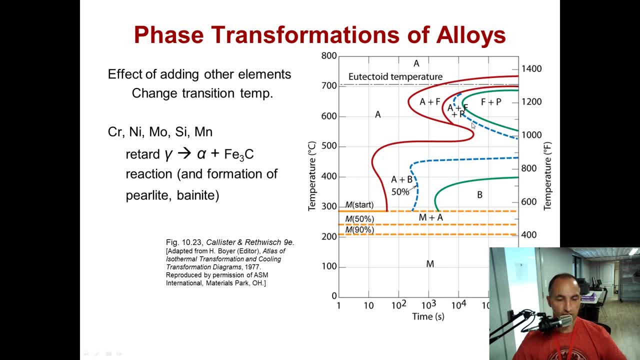 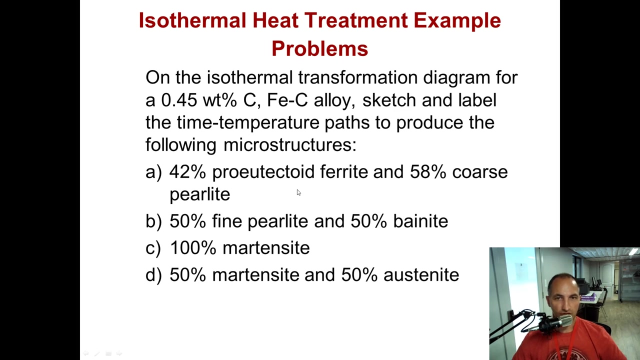 curves to the right so it delays the transformation of austenite to bainite, ferrite and cementite and you also get like a double nose- excuse me, you also get a double nose of that of the isothermal transformation, isothermal heat treatment. example problems. here are four example problems. 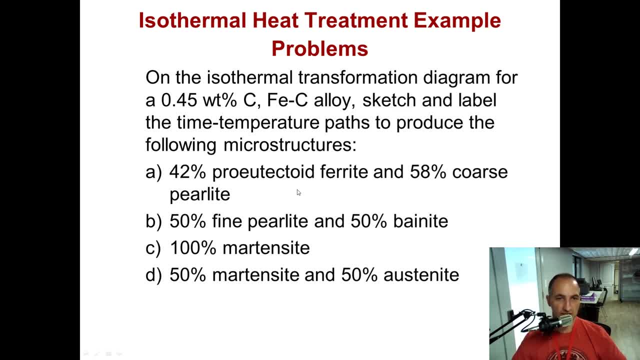 we're taking isothermal transformation diagram of 0.45 weight percent carbon, so this looks like hypo-eutectoid steel because it's below 0.76 and we want to sketch and label the time temperature paths to produce the following microstructures. so let's look at a first: 42% pro-eutectoid ferrite and 58% coarse. 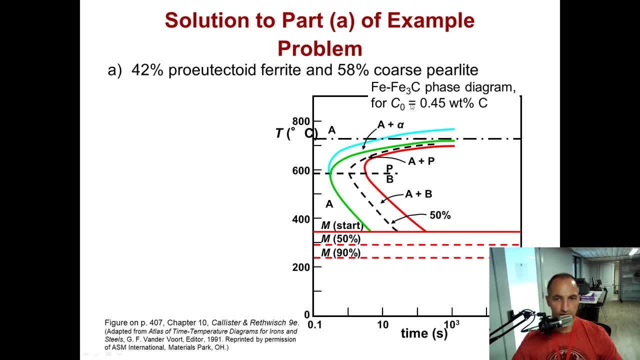 pearlite. so here's our isothermal diagram. here you're pro-eutectoid, which means we have a pro-eutectoid alpha. that's this area here at the top of the nose and let's do this isothermal treatment. so that's the blue line, so we're we're. 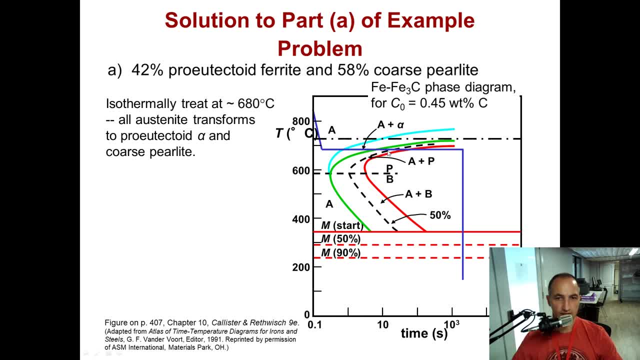 forming the pro-eutectoid alpha here and then it's going into this coarse pearlite. it's at the high end of the pearlite area, so that's going to be. that's why it's coarse pearlite. it's taking a lot longer to form that pearlite. 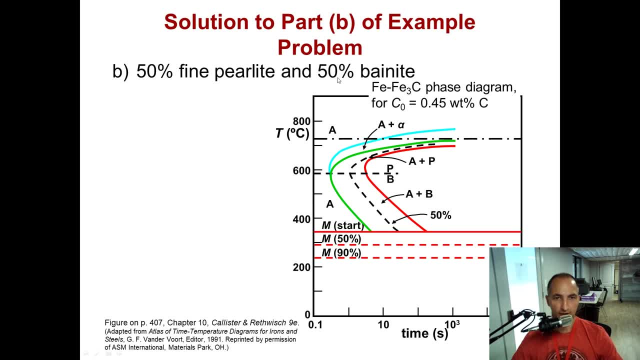 now let's look at 50% fine pearlite and 50% bainite. so fine pearlite. that means we have to go a lot closer to the pearlite to bainite nose here to form that pearlite much more rapidly, which makes it fine and we have to miss the 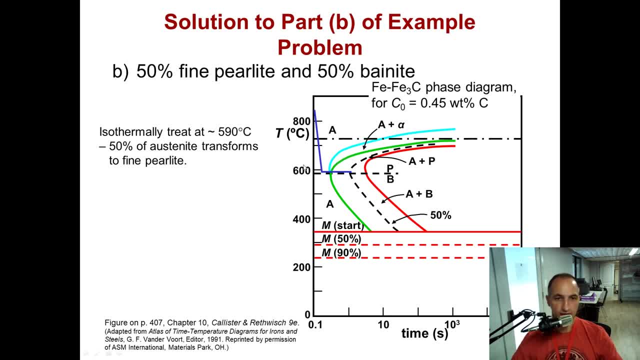 alpha ferrite nose here, and that's why we're we're doing it right down here, here. that here the nose of the transformation diagram. and then we then isothermally treat at 470 to convert all the remaining austenite to bainite, because we have, we've only reached the 50%. 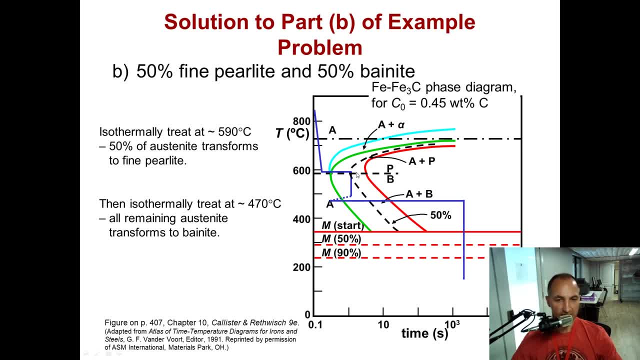 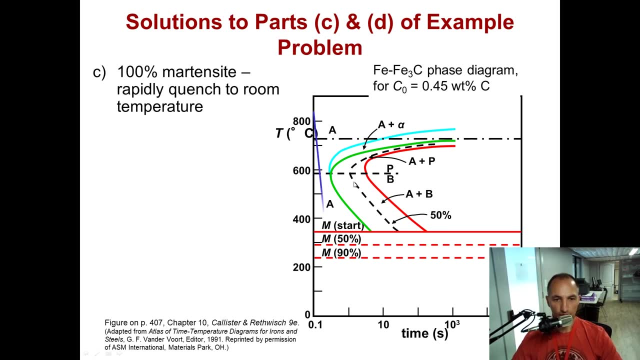 mark here the pearlite, so that means the rest of it is still austenite and we're going to see that in two percent of theernen hair. so we're going to see that Korean tucked here bainite, that is the middle's OUR bainite. 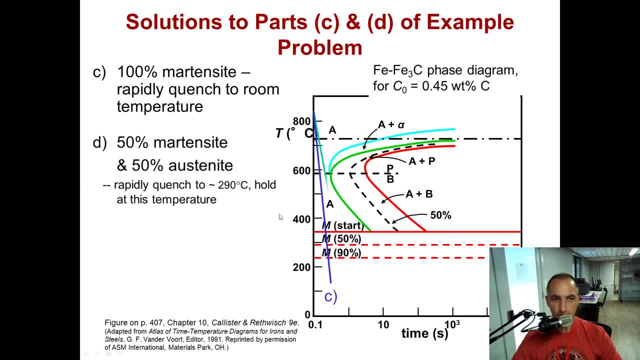 c pink. הנじゃ 자 펀치 어�arthenite. SO THEN WHEN WE QUENCH THAT WE'RE GETTING THE 50% Bainite, let's look at EXAMPLE C, WHICH IS A HUNDRED percent martensite. 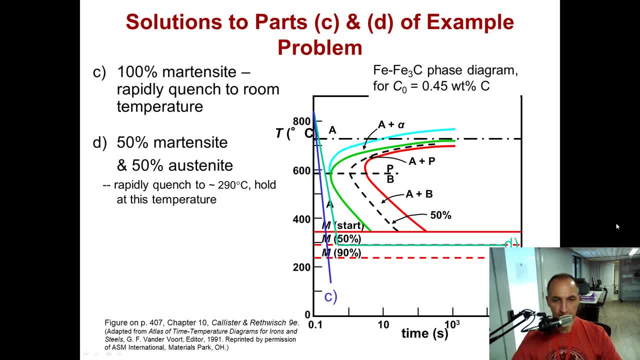 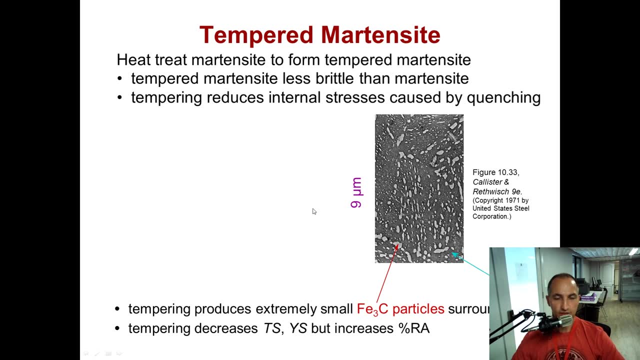 THIS ONE IS KIND OF EASY martensite, and we're just leaving it there at that temperature and holding it at 290 degrees c. so what does tempered martensite look like? as you remember, we had that quenched martensite which is hard and brittle, and then we quench it, and so the those whiskery needles have are you? 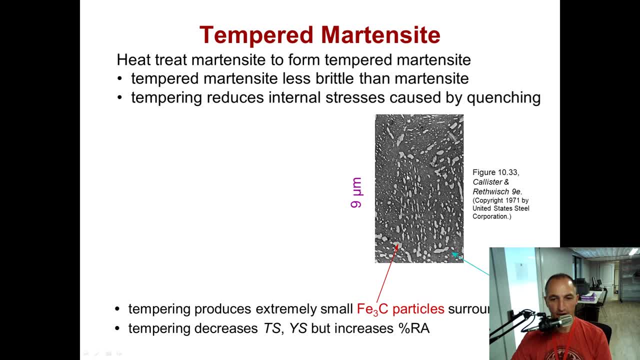 know gone. and you have these iron carbide particles surrounded by this like dark gray alpha ferrite, and this reduces the internal stresses caused by quenching and we get a decrease in intense strength, um and the and uh, and yield strength, but a much greater percent reduction, much greater. 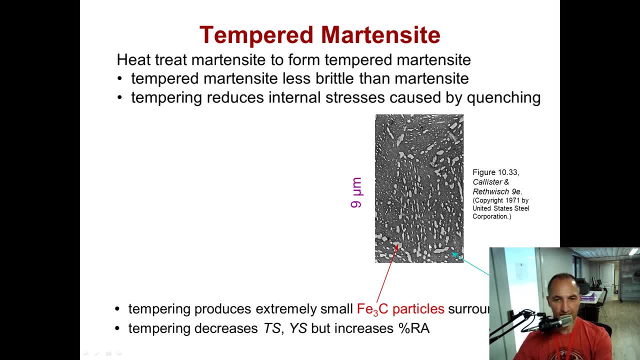 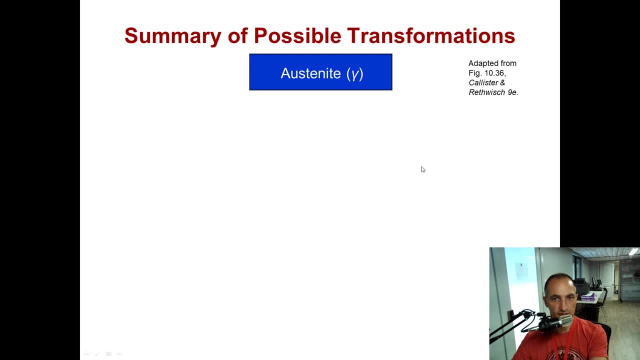 increase in percent, reduction in area. so that's our ductility measurement there. so here's the summary of the possible austenite transformations. we can either do a slow cool, in which case we're going to get perlite. remember that those are the platelets of ferrite plus.